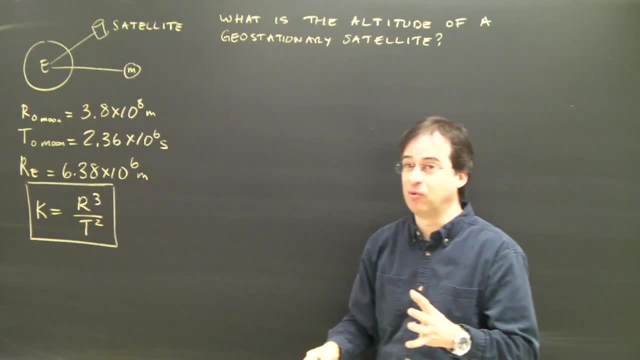 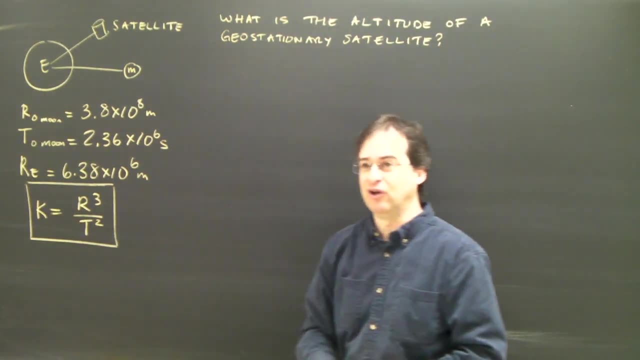 So I'm looking for the altitude. The word altitude is very important. It means what I'm really asking is: what's the height above the surface of the Earth? Okay, so we look at Kepler's third law, And I don't have the constant. 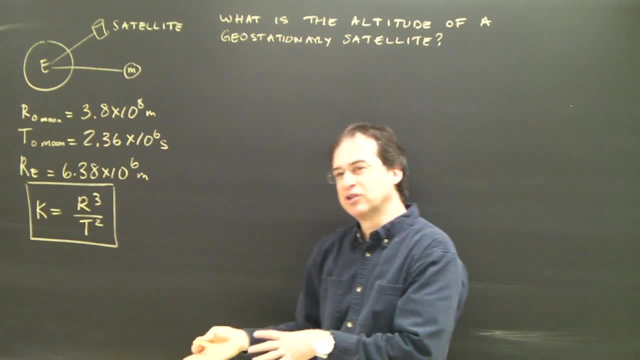 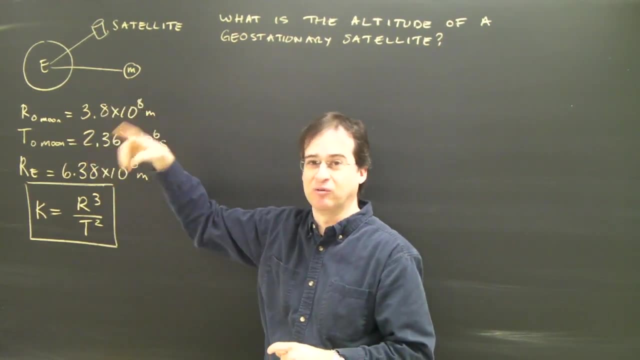 For objects going around the Earth. But I know every object going around the Earth has that same constant, so I can compare one object to another. Like I can say: let's look at the Moon, it's going around the Earth. And let's look at the satellite, it's going around the Earth. 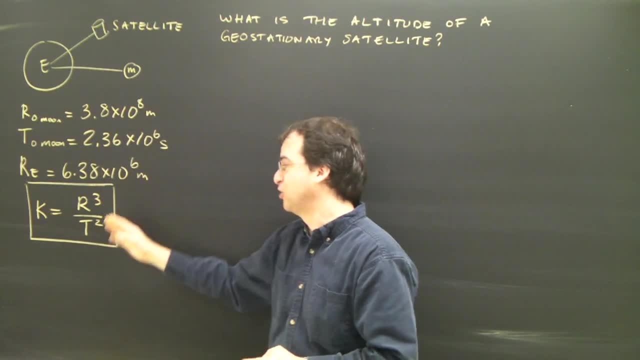 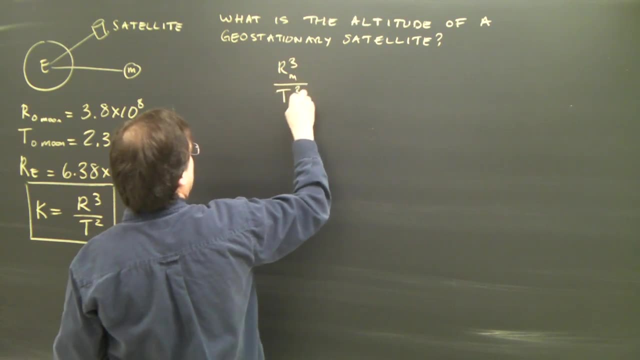 So R cubed over T squared for the Moon should be equal to R cubed over T squared for the satellite. So that's what we're going to do. We're going to say R cubed for the Moon over T squared for the Moon is equal to R cubed of the satellite over T squared. 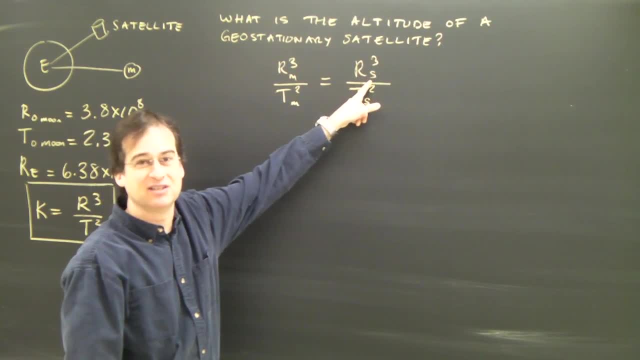 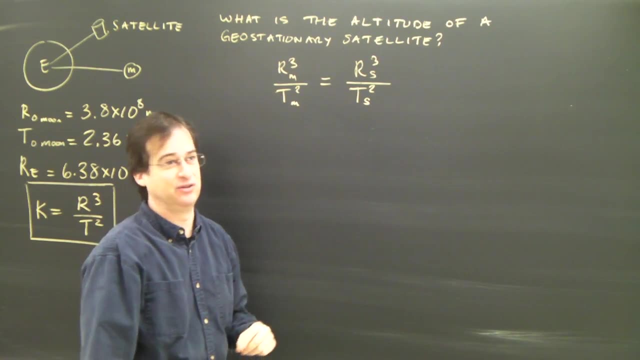 And what we're going to be able to do is solve for the distance to the satellite from the center of the Earth, And then what we've got to do is subtract the radius of the Earth to find out what the altitude is. So let's plug in our numbers. 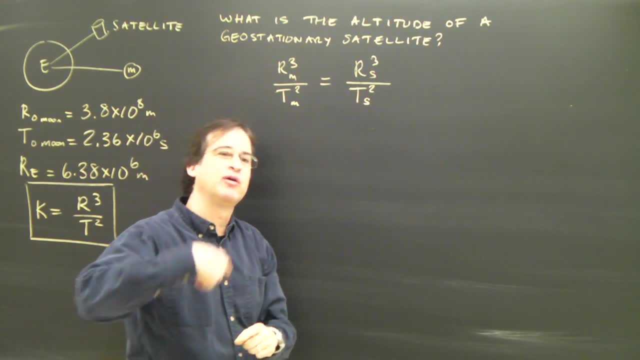 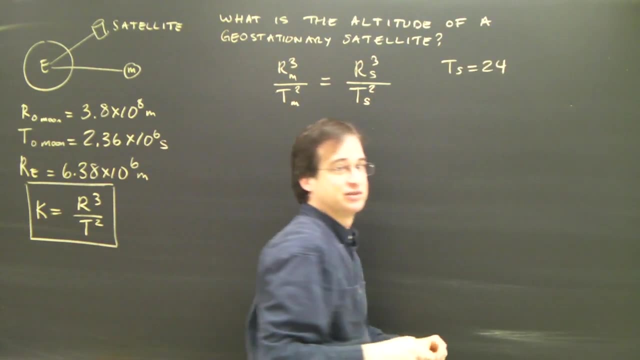 Well, the period of the satellite is going around the Earth once every 24 hours, once a day. So the period of the satellite is equal to 24 hours. But we've got to turn that into seconds. So we multiply by 60 to give us minutes. 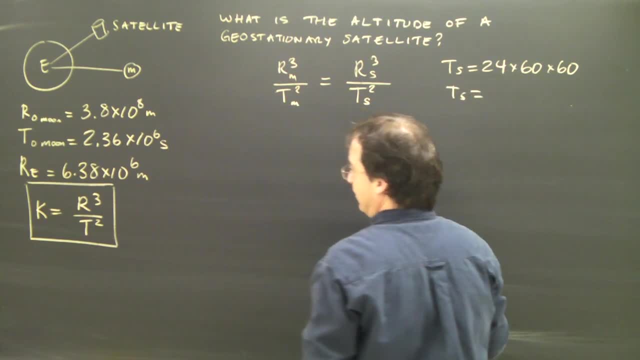 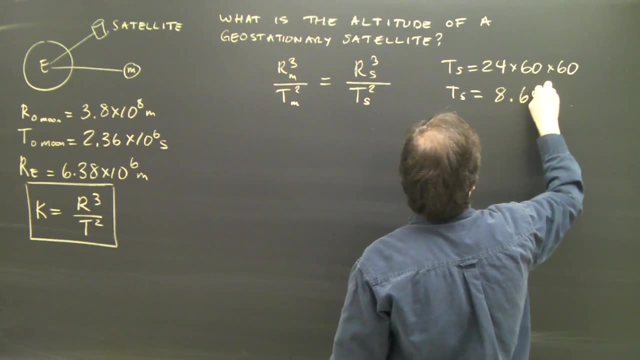 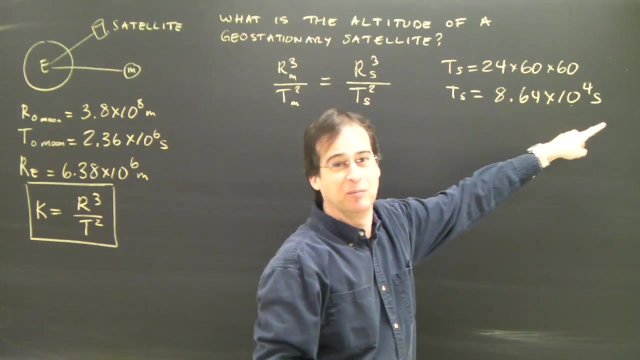 Times 60, the period of the satellite is 8.64 times 4 seconds. So 24 times 60 times 60 gives me that number. That's the period of the satellite in seconds. So let's plug all our numbers here. 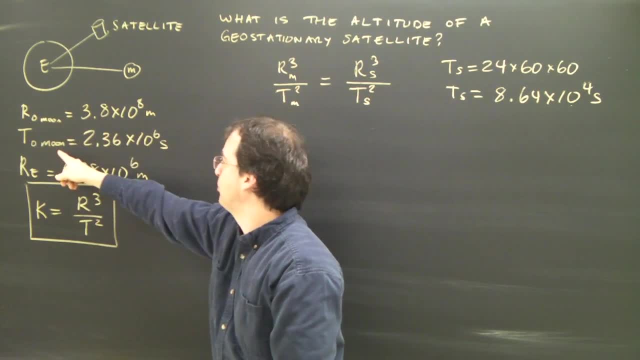 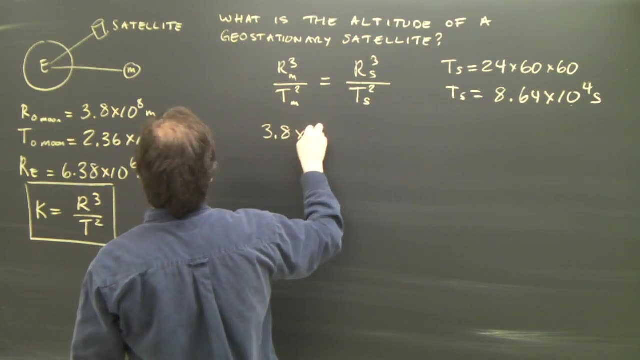 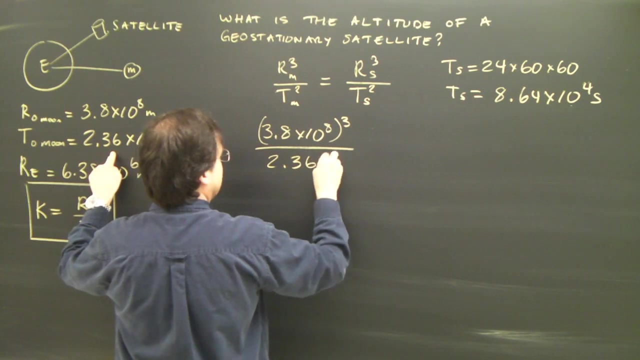 We know the radius of orbit for the Moon. that was given. We know the period of the Moon in seconds And we're going to use this one later, So we got it. We've got 3.8 times 10 to the 8th cubed over 2.36 times 10 to the 6th squared. 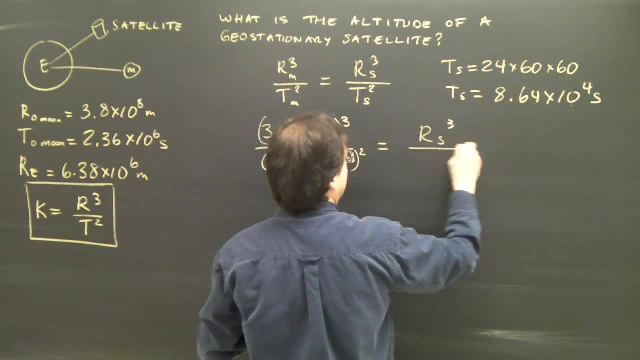 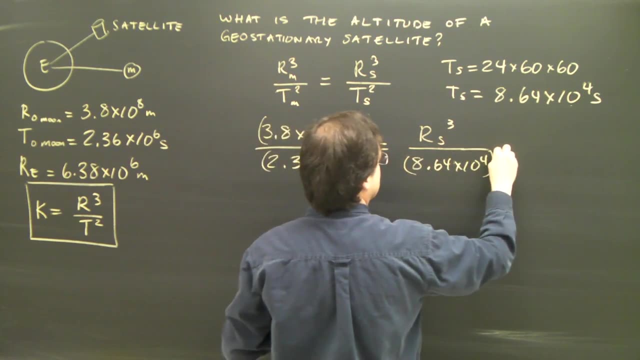 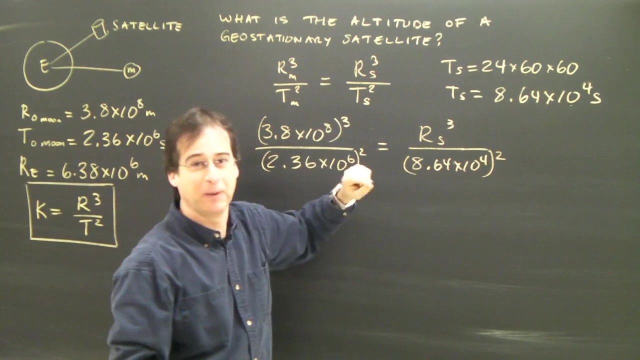 equals what we're looking for. raise the satellite, divided by 8.64 times 10, to the 4th and that is squared. So I've got everything in my formula. Remember to cube this square. that That's a cube, that's a square.